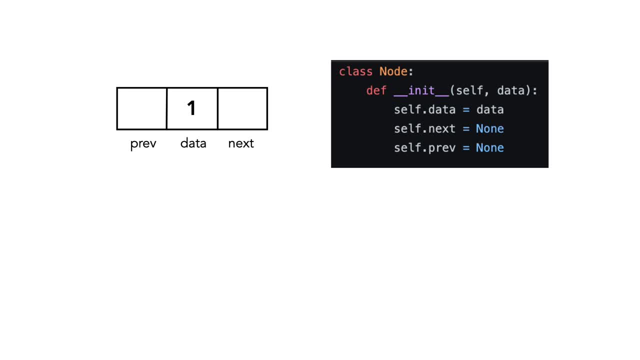 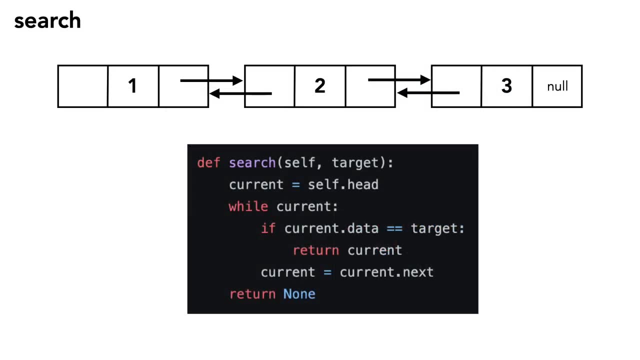 Data. next and previous. The list starts with no object, So the head pointer points to null. The first operation I want to discuss is search. Let's use the following list and search for the node with the data value of 3.. 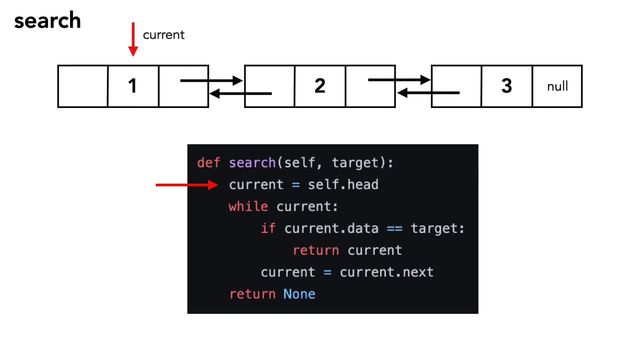 We set a current node equal to the head of the linked list. While current is not null. we iterate through the list, comparing the data of the current node to our target. If they match, we return the current node. Otherwise, we set current equal to the current's. next. 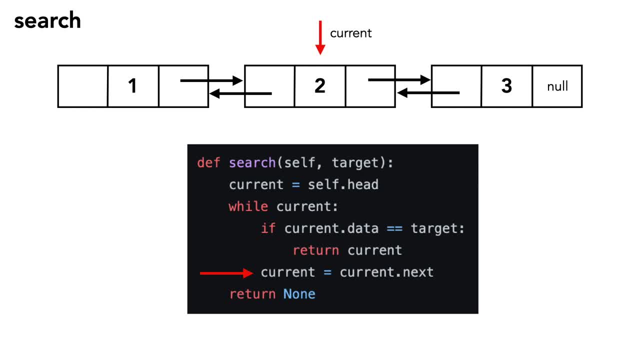 In this example, we pass over 1 and 2 until we get to the third node, where the data is equal to our target. In the worst case, we'll visit every node in our list. So time complexity is O. Let's discuss inserting a node at the front of our list. 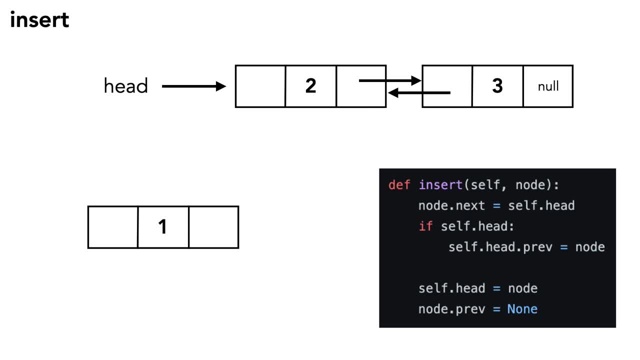 We want to insert the object on the left that has a data value of 1.. Let's follow the code on the right. First, we set the node's next pointer, equal to the head object. Next, we set the head object's previous pointer equal to the node. 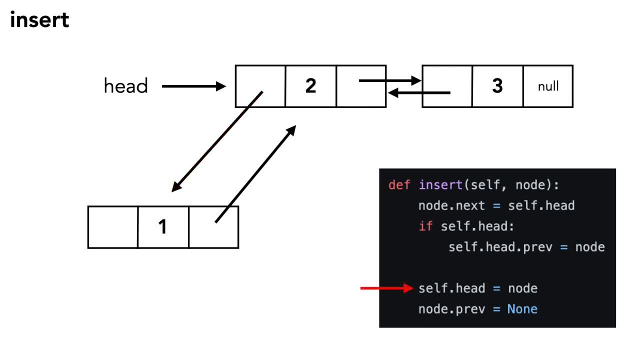 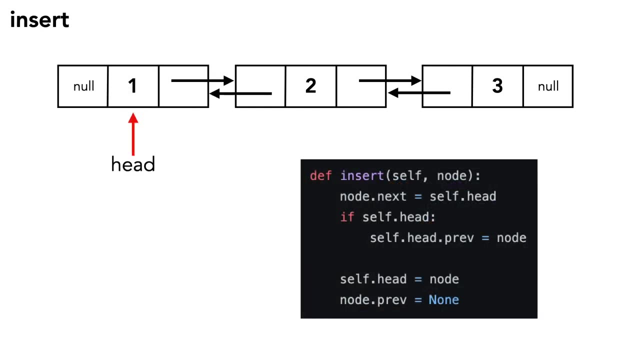 We then set the head pointer to the recently added node. Lastly, we set the node's previous pointer to null. Our node is now added into the list. This is a constant time operation, so it has a runtime of O. Finally, let's discuss deleting a node from a linked list. 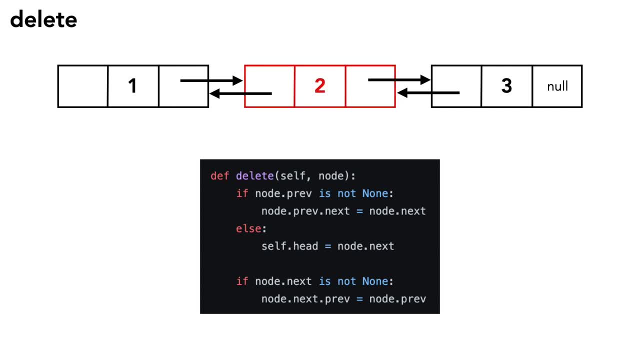 In this case, we want to delete the node with a data value of 2.. The node we want to delete has a previous pointer that points to 1. We set 1's next pointer to 2's next node. 2's next node is 3.. 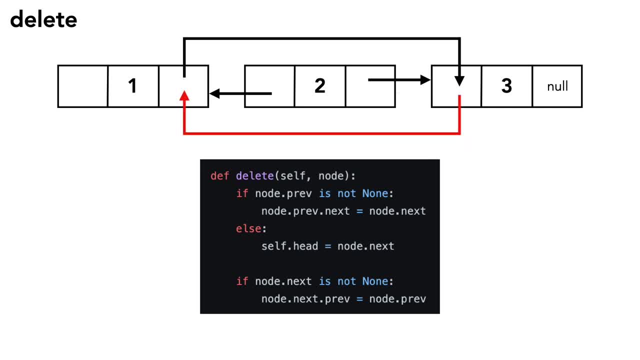 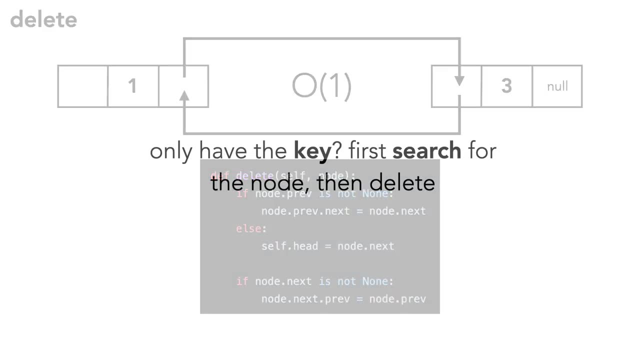 We set 3's previous pointer to 2's previous pointer, which is 1.. Similar to insert. this is a constant time operation, so its runtime is O. However, if you only have the key, which was 2, and not a pointer to the node, 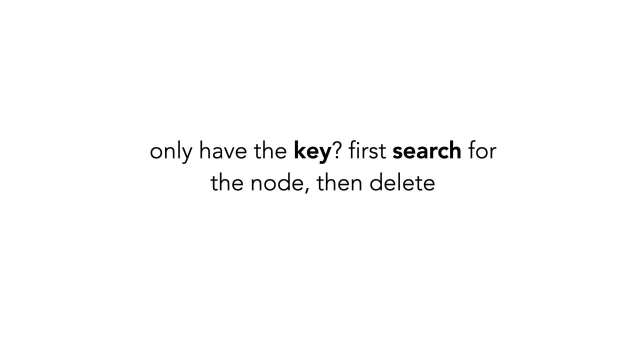 you first need to search the list which, as we discussed earlier, is O. Thank you for watching. Please subscribe and share. 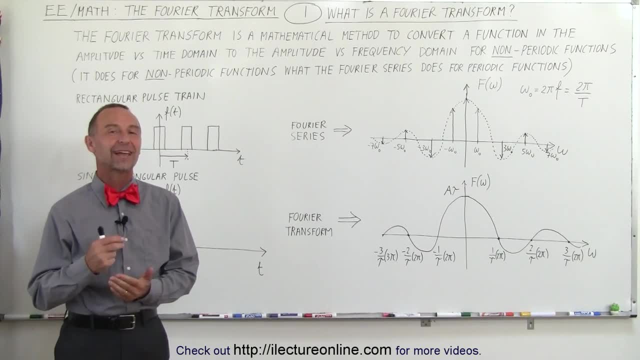 Welcome to Electron Line. Here we're starting a new series, This time a series. Let's try again: The Fourier transform. That's the series we're going with. Yep, all right, Welcome to Electron Line. Here we're starting a new video series on the Fourier. 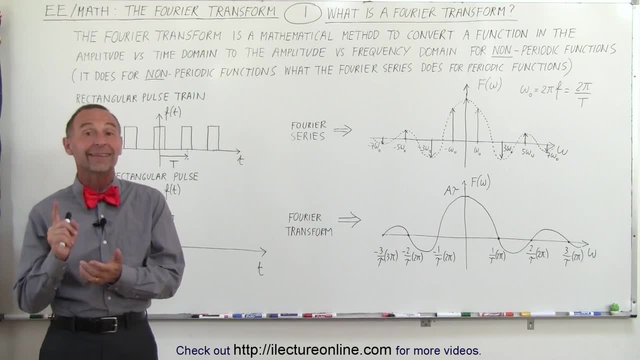 transform. Now there's a lot of similarities and a lot of dissimilarities between the Fourier transform and the Fourier series. So let's read the definition Now keep in mind it's going to take a few videos to get a real good appreciation of what the Fourier transform actually is. 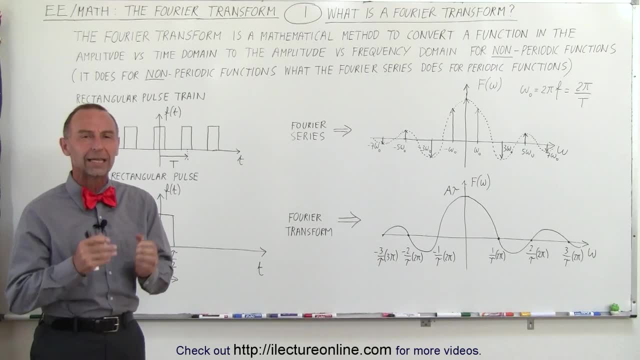 Maybe after about five or ten videos or so, we'll have a fairly good understanding. We need to understand its behavior, how it's used and why do we need the Fourier transform. Well, first of all, let's read the definition and see what it says. 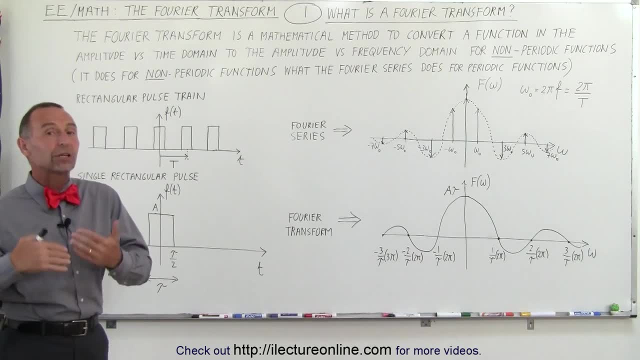 The Fourier transform is a mathematical method, Just like the Fourier series. it's a mathematical method to convert a function in the amplitude versus time domain to the amplitude versus frequency frequency domain. well, that sounds an awful lot like the Fourier series, because that's exactly 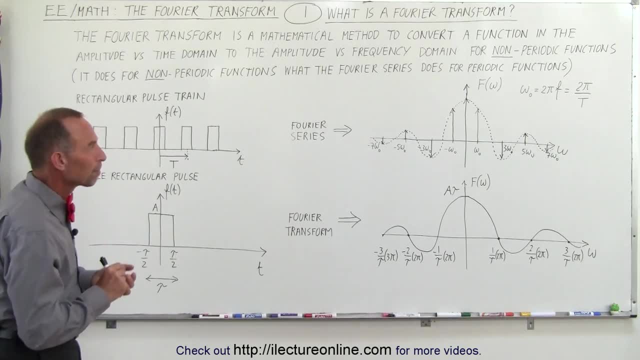 what the Fourier series does, but there's one big difference: the Fourier series works on periodic functions, and so the question is: what do we do when we have a non-periodic function? and it turns out the Fourier transform does exactly what the Fourier series does, but it does so for non-periodic